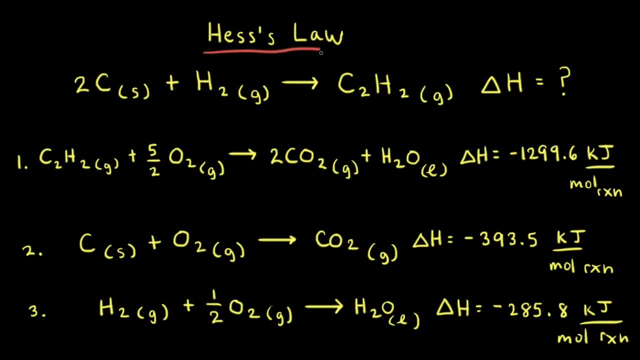 Hess's law states that the overall change in enthalpy for a chemical reaction is equal to the sum of the enthalpy changes for each step, And this is independent of the path taken, so it doesn't matter what set of reactions you use. 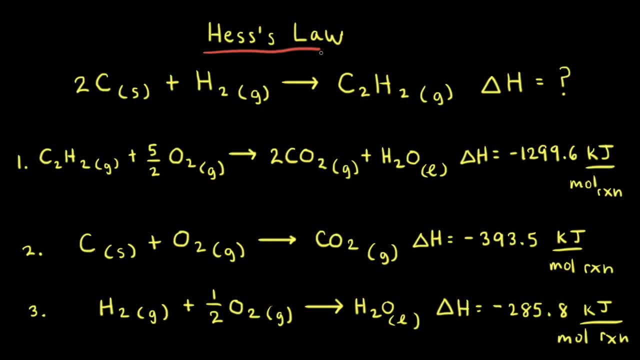 If you add up those reactions and they equal the reaction that you're trying to find. you can also sum the enthalpies to find the enthalpy change for the reaction. As an example, let's say we're trying to find the change. 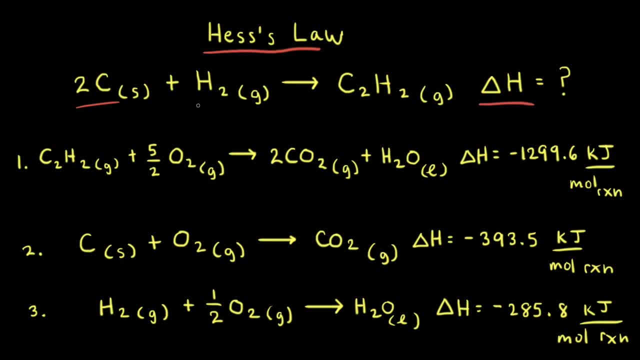 in enthalpy for the reaction of carbon with hydrogen gas to form C2H2, which is acetylene. We can calculate the change in enthalpy for the formation of acetylene using these three reactions below. Our approach will involve looking at these three reactions. 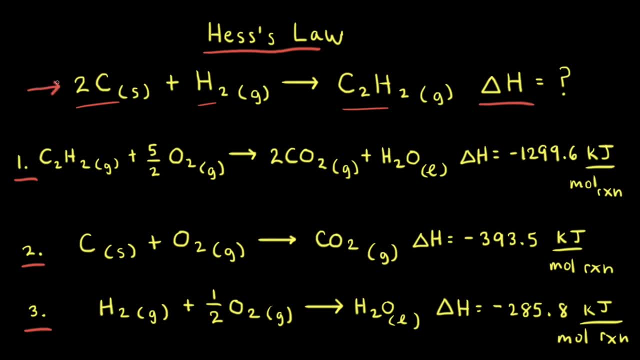 and comparing them to the original reaction to see if we need to change anything. For example, if we look at reaction one, there's one mole of acetylene on the left side of the equation And if we compare that to the original reaction, 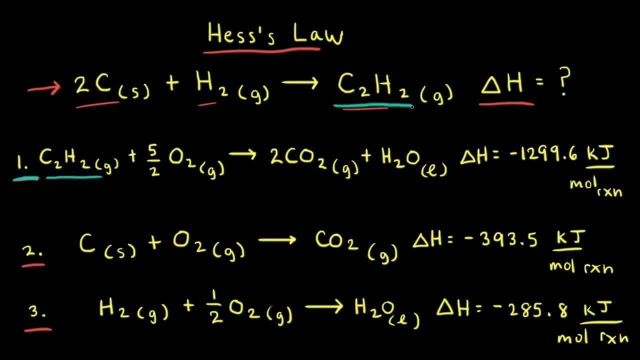 there's one mole of acetylene on the right side of the equation, So we need to reverse equation one to make it look more like our original reaction. To save time I've gone ahead and reversed equation one, So you can see I did that down here. 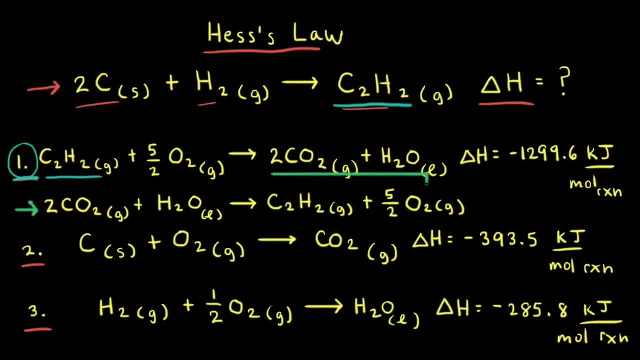 Looking at the original equation, for equation one, here were the products, and now we've made those products the reactants. And what were the reactants over here? for equation two, And what were the reactants over here for equation three, And what were the reactants over here for equation four: 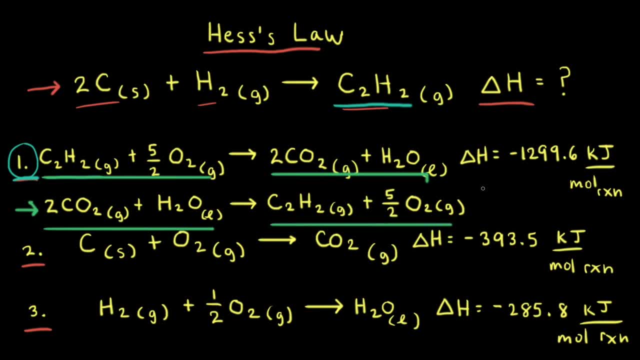 And what were the reactants over here? for equation one have now become the products. The change in enthalpy for equation one is negative: 1,299.6 kilojoules per mole of reaction. Kilojoules per mole of reaction just means: 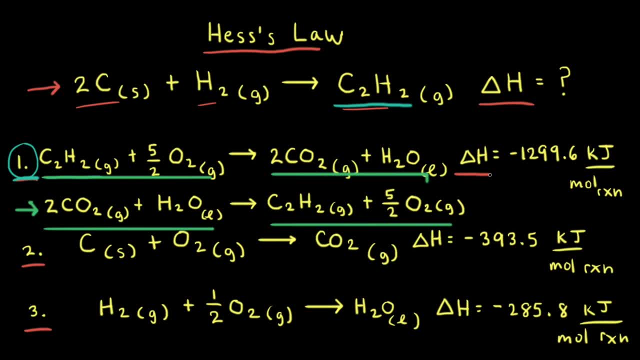 how the reaction is written in the balanced equation. And since we've reversed equation one, we also need to reverse the sign for delta H. So, instead of this being a negative, instead of this being a negative, we're gonna go ahead and change this into a positive. 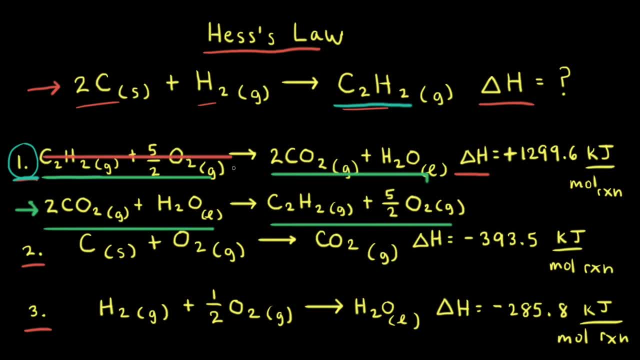 And also let's go ahead and cross out the first equation so we don't get confused. Next we look at equation two and we compare it to our original. For equation two, there's one mole of solid carbon on the left side And looking at our original reaction, 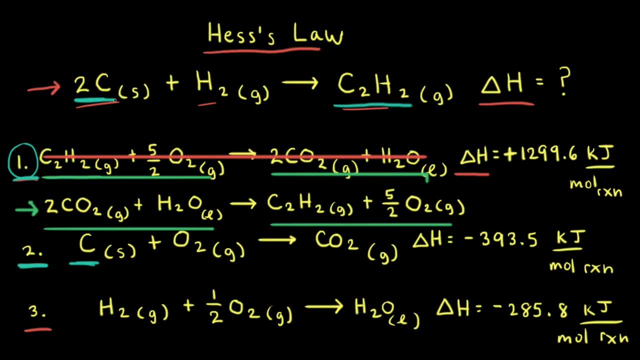 there's two moles of carbon on the left side. So to get equation two to look like our original equation, we need to multiply everything through by a factor of two. So we're gonna multiply everything in equation two by a factor of two. 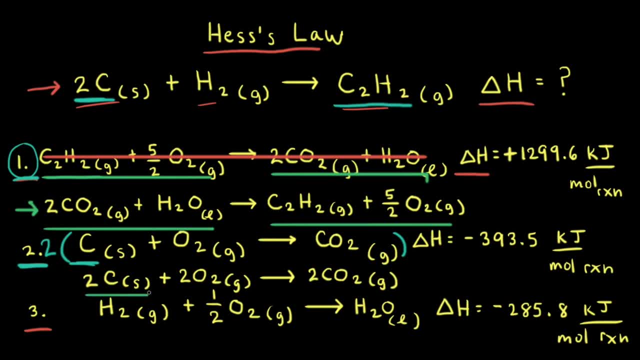 To save some time, I've gone ahead and written out what we would get. We would get two carbons plus two O2s. goes to two CO2.. The change in the enthalpy for the formation of one mole of CO2 was negative: 393.5 kilojoules. 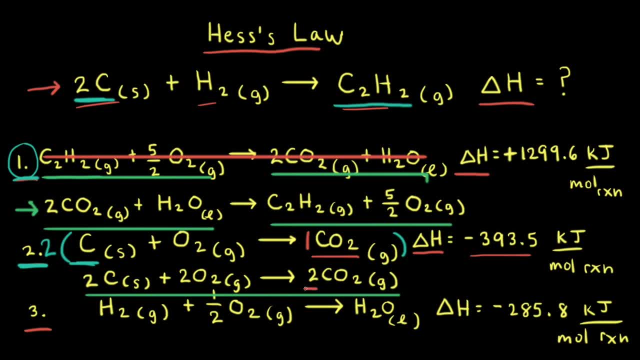 per mole of reaction, But now we're forming two moles of CO2.. And since we multiplied the equation through by a factor, we also need to multiply the change in enthalpy by a factor of two as well. And also, let's go ahead and cross out this first version here. 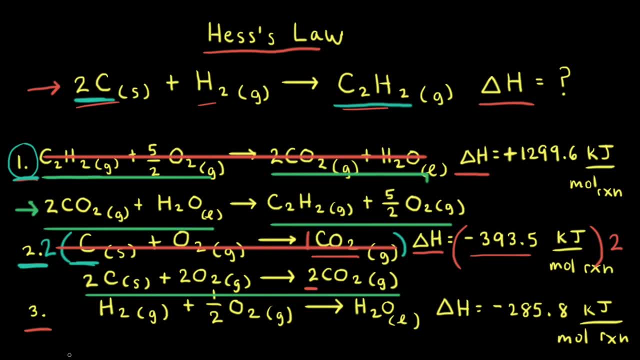 because now we're forming two moles of CO2.. Next we look at equation three and we can see there's one mole of hydrogen gas on the left side of the equation which matches the original reaction, which also has one mole of hydrogen gas on the left side. 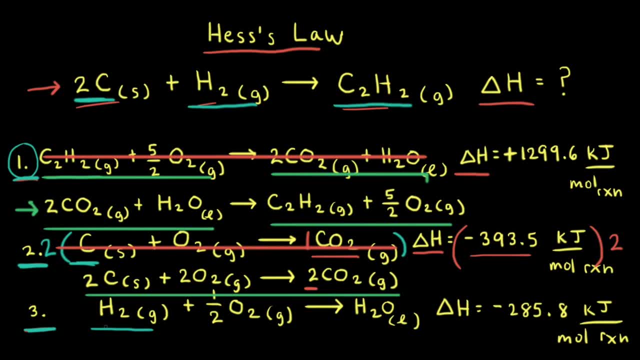 So we don't need to do anything to equation three And since we're not doing anything to the equation, not going to do anything to the change in the enthalpy, so it's going to stay negative: 285.8 kilojoules per mole of reaction. Next we add up all of our 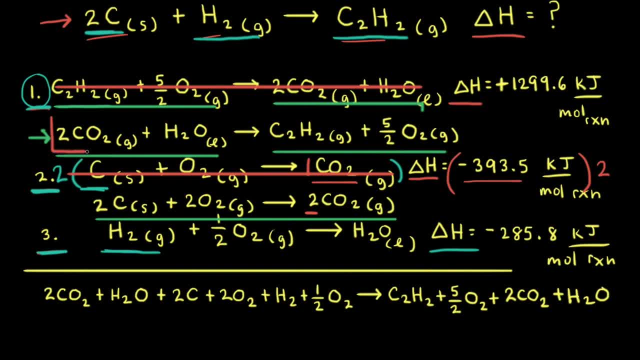 reactants and products. So we have 2 CO2 plus H2O plus 2 C plus 2 O2 plus H2 plus 1 half O2, so those are all written down here for our reactants And then for the 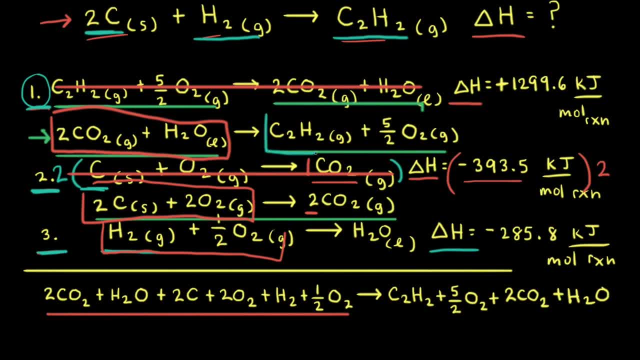 products. let me just change colors. here we have C2H2 plus 5 O2 plus 2 CO2 plus H2O, and so those are written over here for the products. Next we see what we can cancel out. There's 2 CO2s on the left side and there's 2 CO2s on the right.